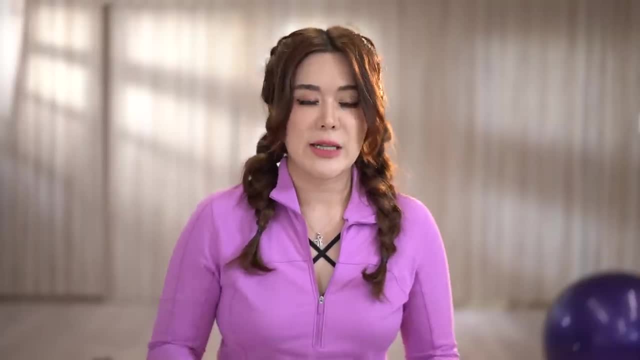 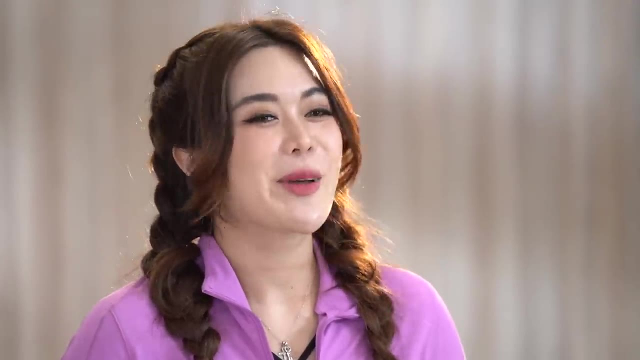 worldwide During this time. absolutely nobody wants to get sick, so you want your own immune system to be working at its full potential. Today, I'd like to introduce you to a very special doctor here at Bumrungrad International. She's an anti-aging and regenerative medicine specialist. 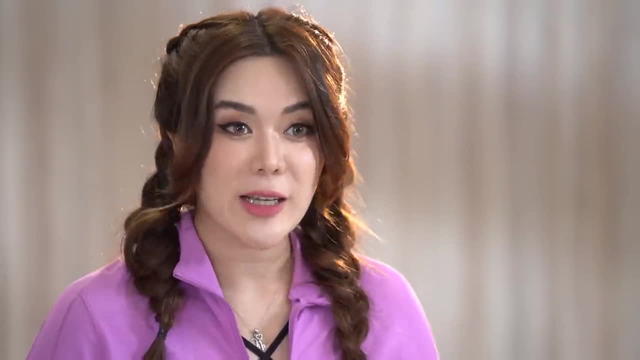 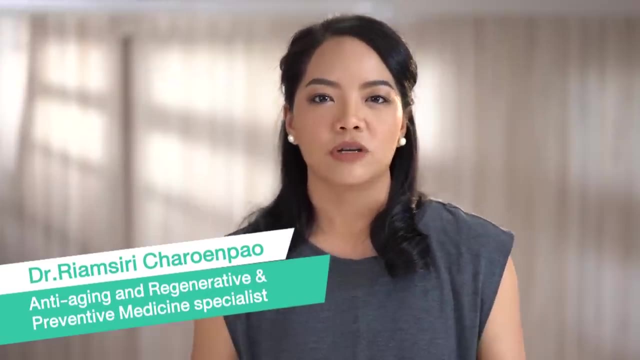 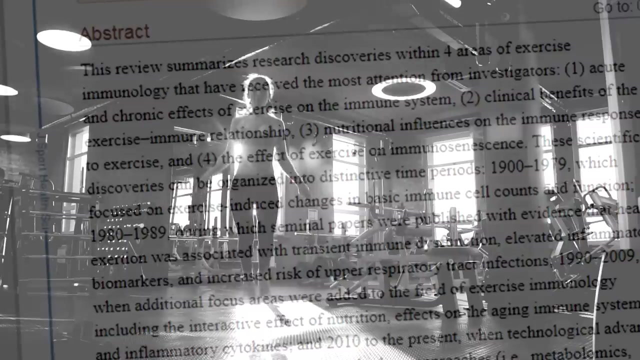 named Dr Ramsari, and today she'll be taking us through an exercise program designed to boost your immune function. Thank you, Dr Amy, for a great introduction. There are several studies that have shown exercise of even less than 60 minutes can improve your immune function. Before we get, 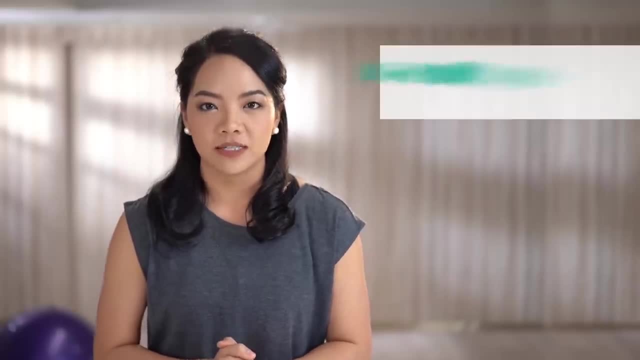 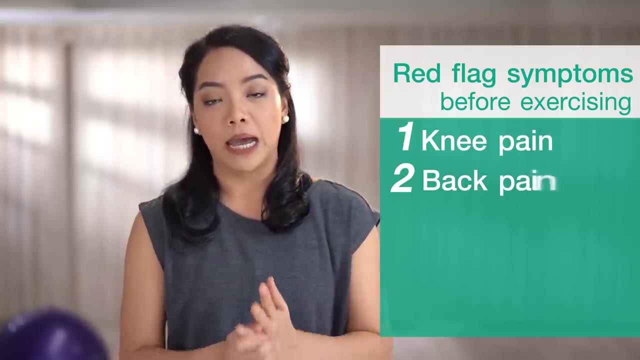 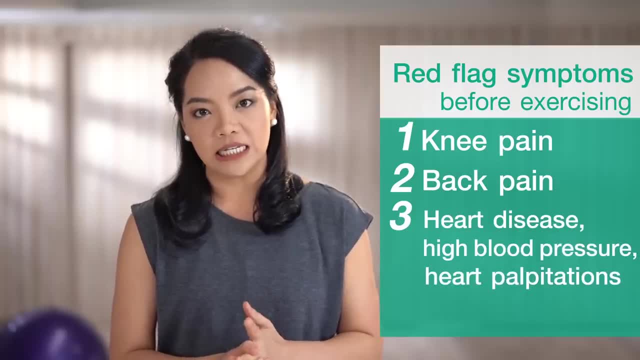 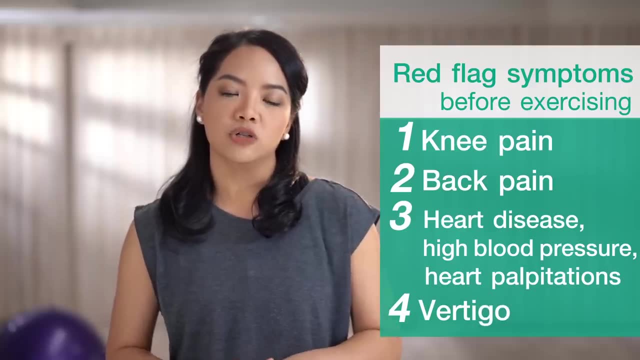 So if you have uninvestigated knee pain, uninvestigated back pain, other preexisting medical conditions such as heart disease, high blood pressure, heart palpitations or history of vertigo, I advise that you talk to your doctor prior to starting these exercises with us. Let's. 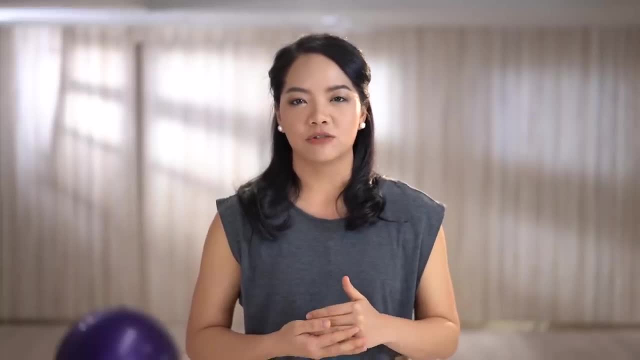 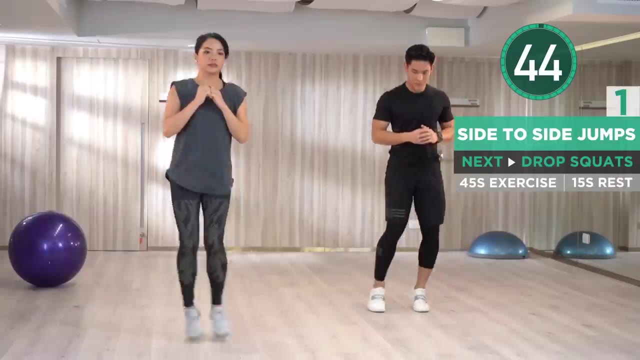 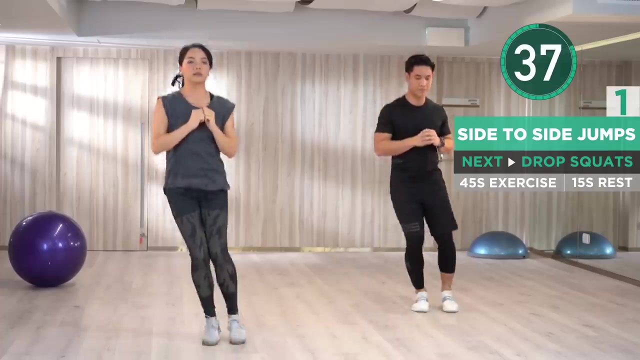 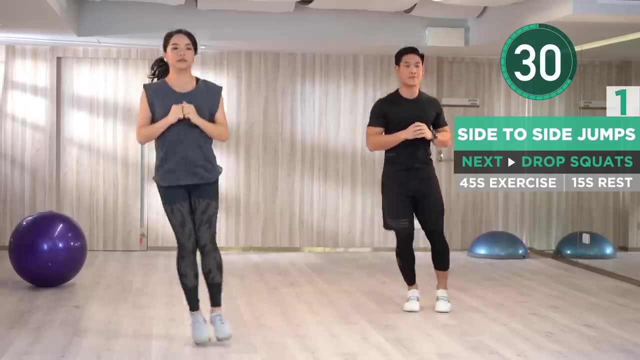 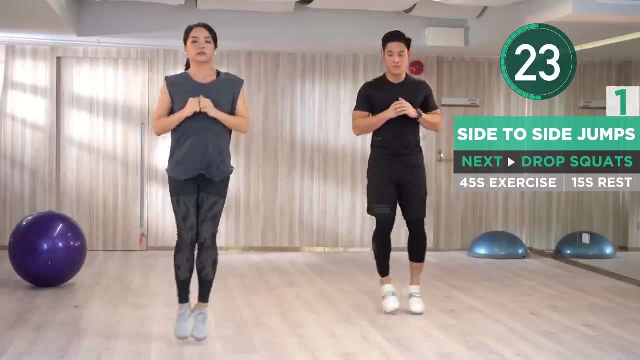 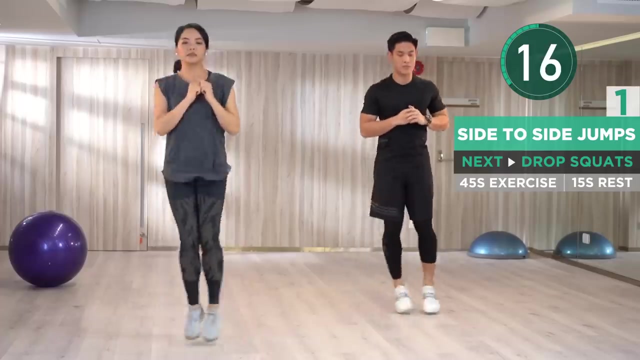 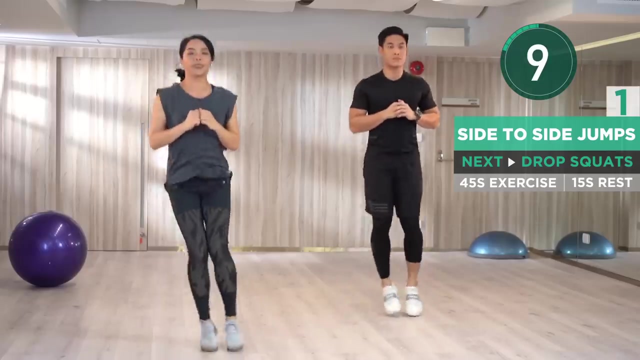 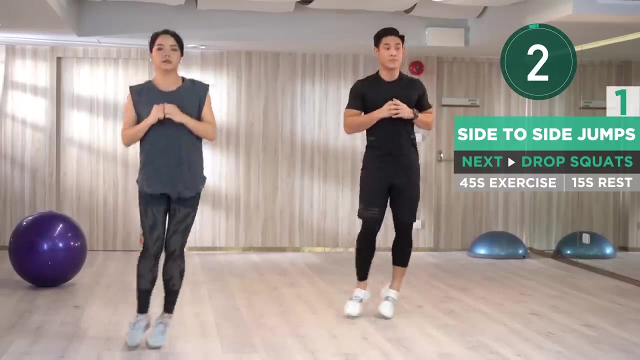 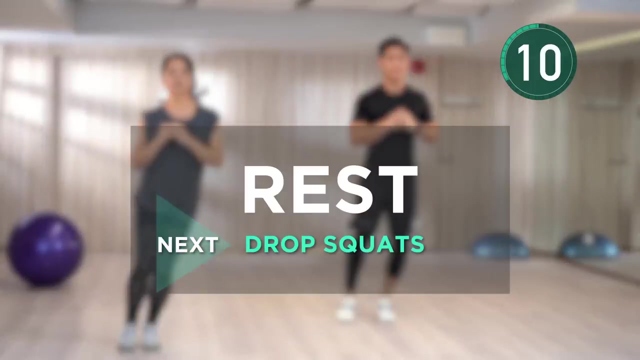 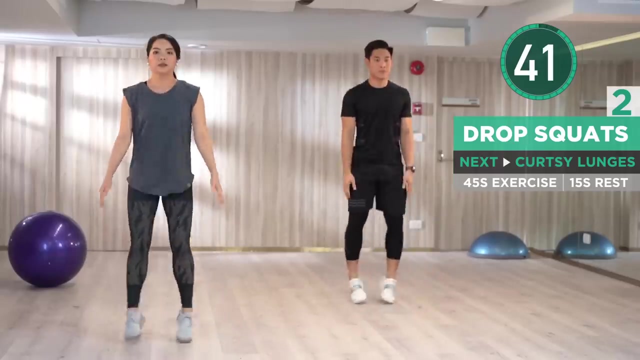 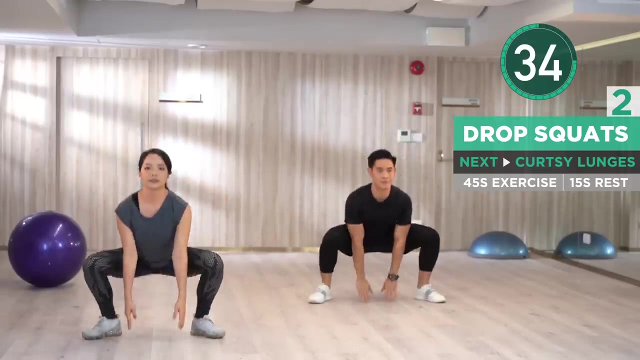 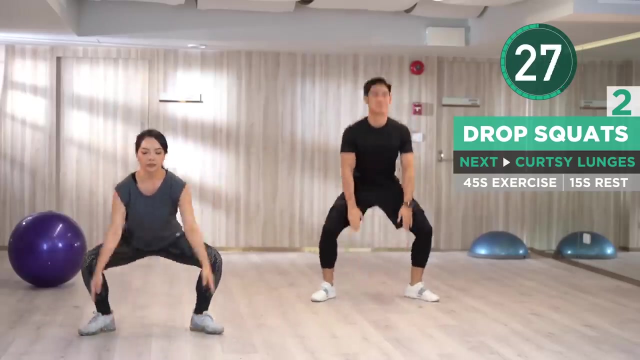 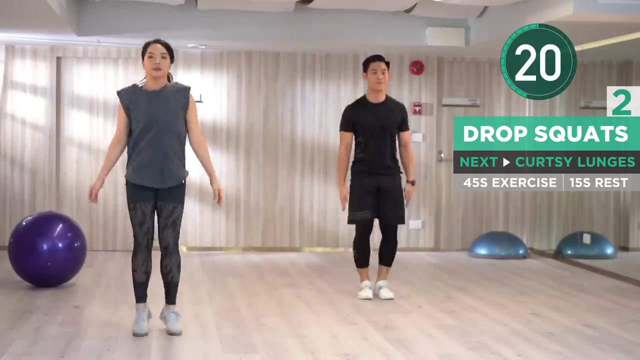 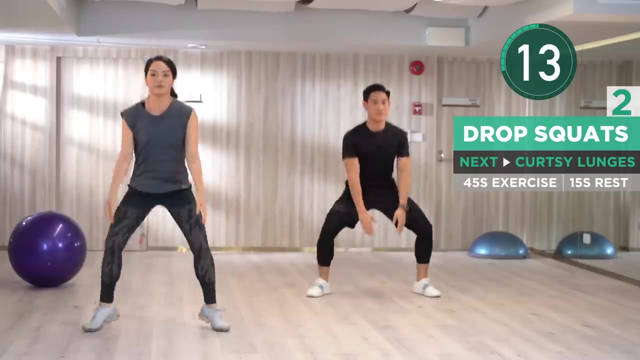 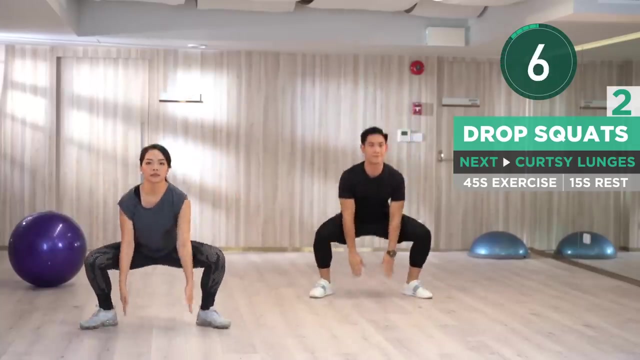 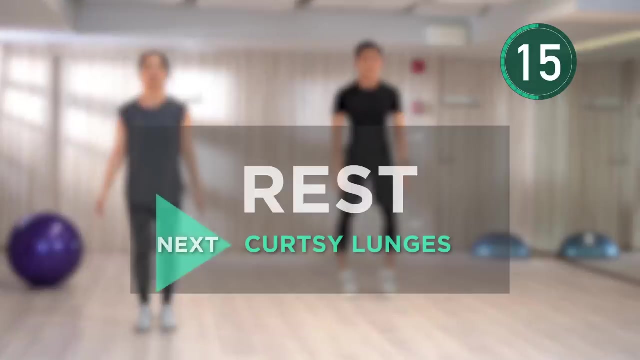 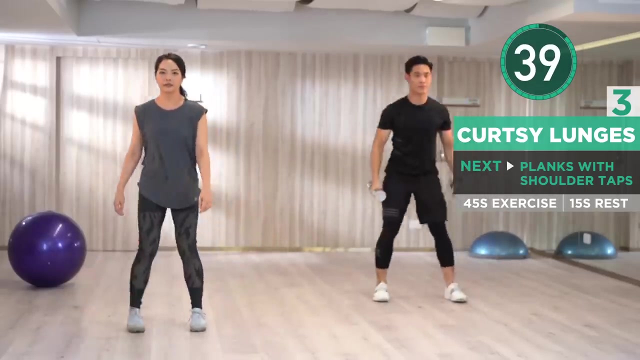 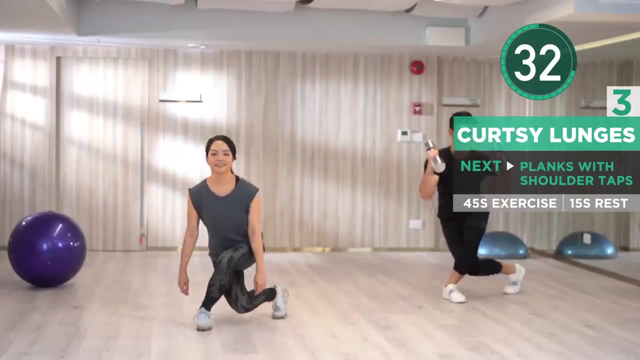 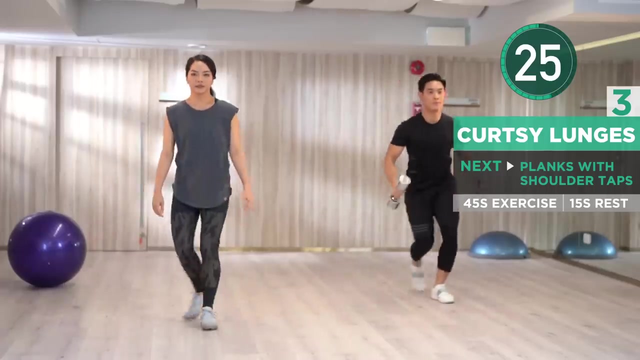 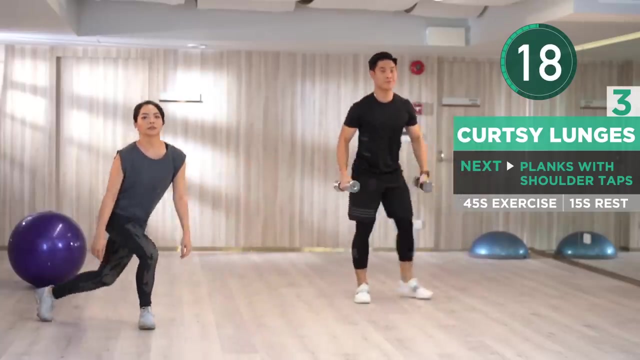 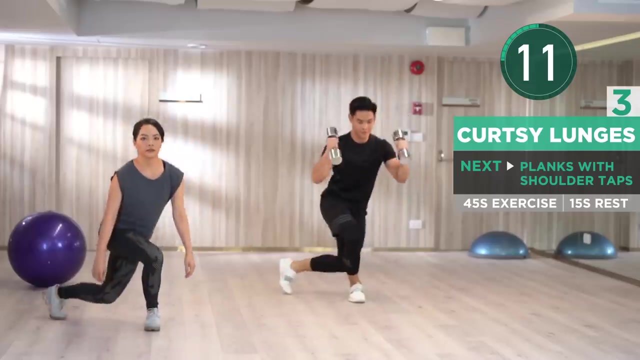 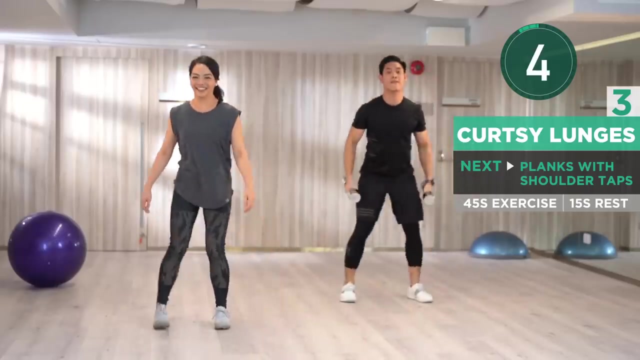 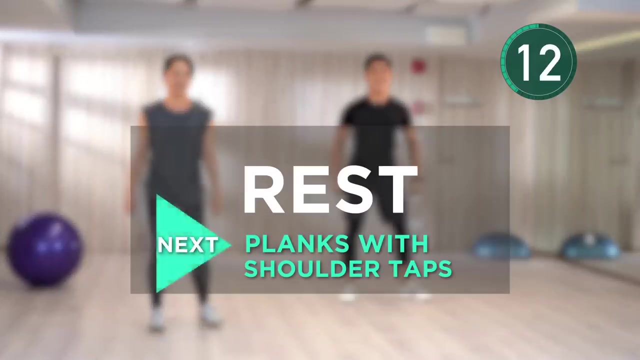